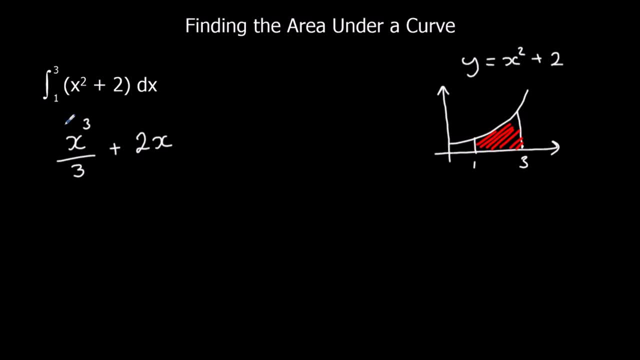 and divide by 1, which I'm not going to do Now. you would usually add c when you're integrating. We don't have to do it when we're doing definite integration. If we did, it wouldn't matter because the c's would cancel anyway. So you'll. 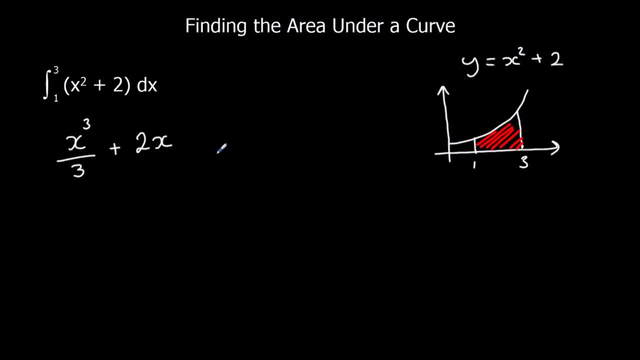 have a c in the first one, a c in the second one, you'll take them away and it will go. So we don't have to add c. So we're going to integrate it now and we're still going to substitute in the 3 and the 1.. 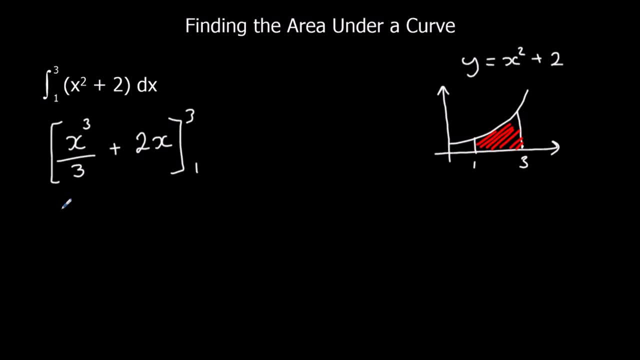 We actually want to add這麼 when we add the 1 to the power, because that makes 2 and that makes 3, so I can get the 1.. However, look, if we had done the 3 over here and we have Allison here, we wouldn't have. 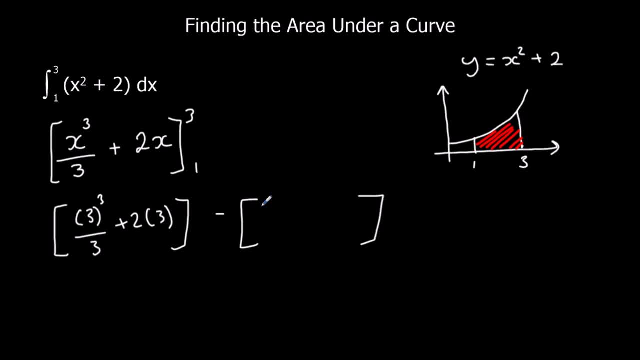 added x squared, So we're going to add 3 divided by 3.. So that would be 2 cubed divided by 3, plus 2 cubed squared 1 times셔야 Prime prove i: at this stage. you just type it into the calculator and it will tell you the. 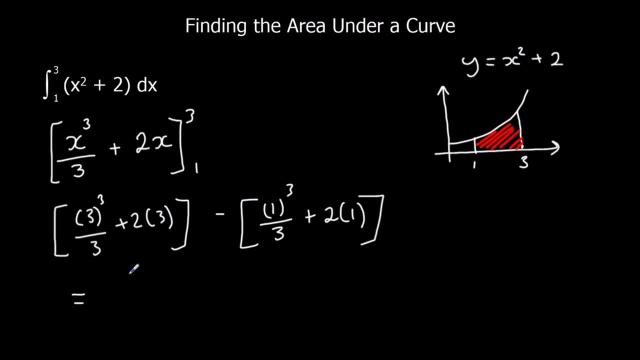 answer. so if we type this into the calculator, we should get 38 over 3 and it's squared, unit squared because we're dealing with area. okay, here's another question. so this time we're being asked to find the area underneath 3x squared plus root x between 4 and 1. so we're going to follow the same process. so 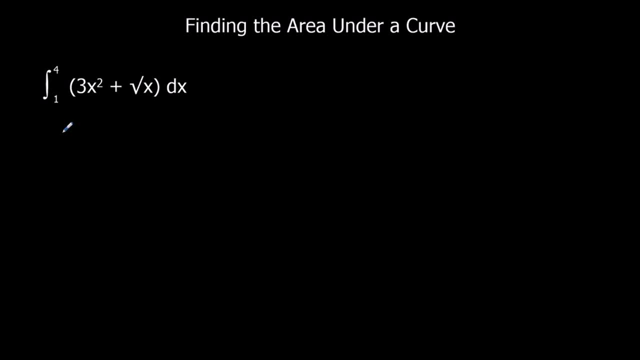 we're going to integrate first. so we're going to add 1 to the power and divide by the new power. so if I add 1 to the power, that's x cubed, and divide by the new power, x root, x is the same as x to the power half. so if I add 1 to the power, 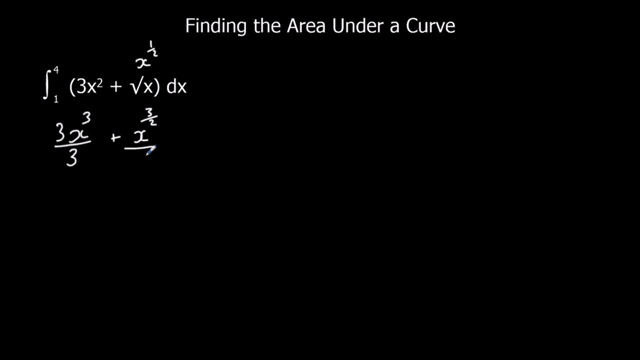 becomes x to the power of 3 over 2 and I'll divide by the new power. again, I'm not going to add C, because when we're dealing with definite integration we don't need to, and I'll put the 4 on the 1 over here. now I can simplify this a. 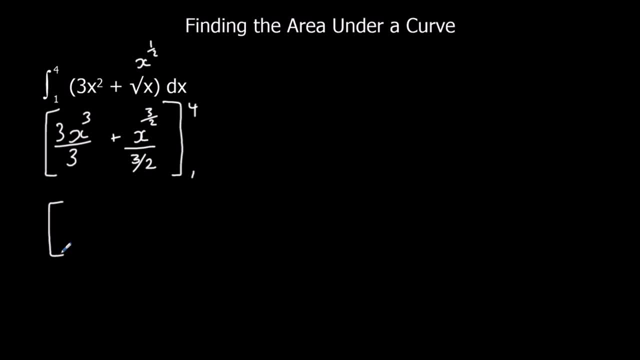 little bit before I carry on, so I'll do that first. so 3 divided by 3, well, the 3 is going to cancel, so that's just x cubed. and if I divide by 3 over 2 that becomes 2 thirds. so I have 2 thirds x to the. 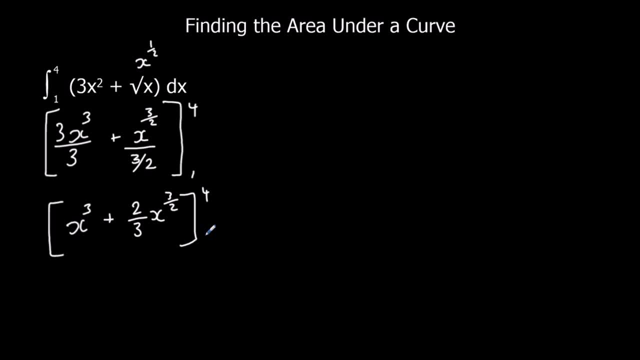 power of 3 over 2. so now I need to substitute in the 4 on the 1. so so I'm going to have 4 cubed plus 2. thirds of 4 to the power of 3 over 2. take away 1 cubed plus 2. 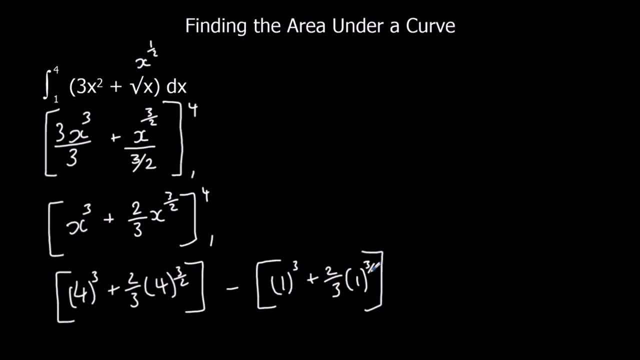 thirds of 1 to the power of 3 over 2. and again we're going to substitute. just type it into the calculator now and we should get out 203 over 3 units squared. okay, here's another question. what we've got to do for this one is we've got to 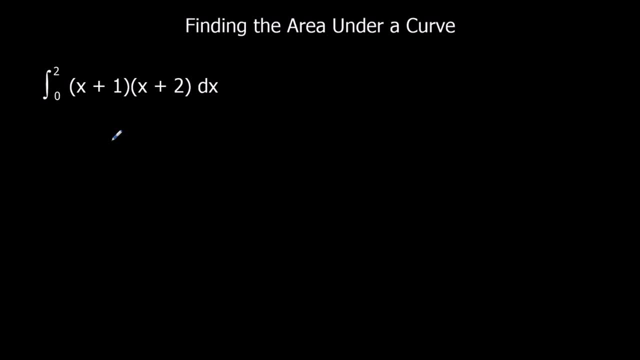 expand the bracket before we can integrate. so if we expand and simplify, you should get x squared plus 3x plus 2. so then we're going to follow the same process we did before we can integrate it. so if I add 1 to the power, 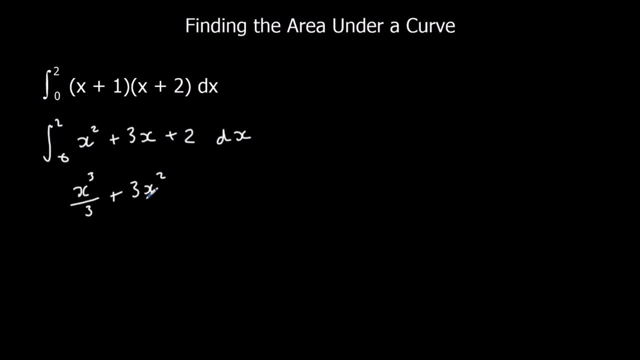 divide by the new power. add 1 to the power divide by the new power: A 1 to the power divided by the new power. I don't have to add c, and then I'm going to substitute in the 2 and the 0, and that will give me the answer. so that's 2 cubed over. 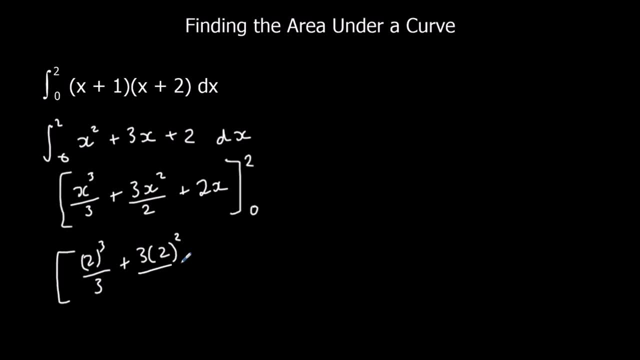 3 plus 3 times 2 squared over 2 plus 2 twos. take away 0 cubed over 3 plus 3 zeros squared over 2 plus 2 zeros. so again we can just type that into the calculator and we should. 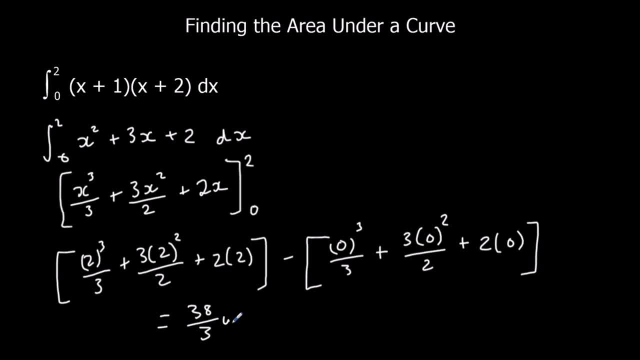 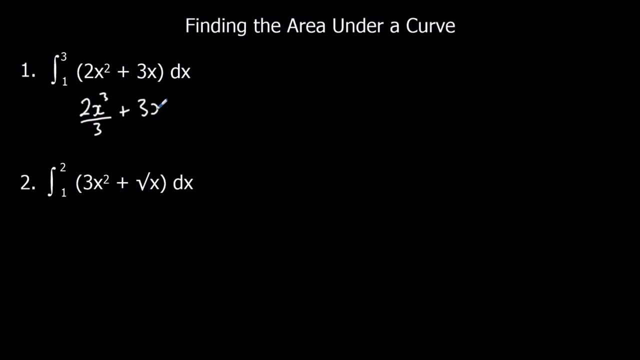 get out 38 over 3.. Okay, here's some questions for you to have a go at. so pause the video, give them a go, and then you can press play after. Okay, first step: integrate. so add 1 to the power divided by the new power. add 1 to the. 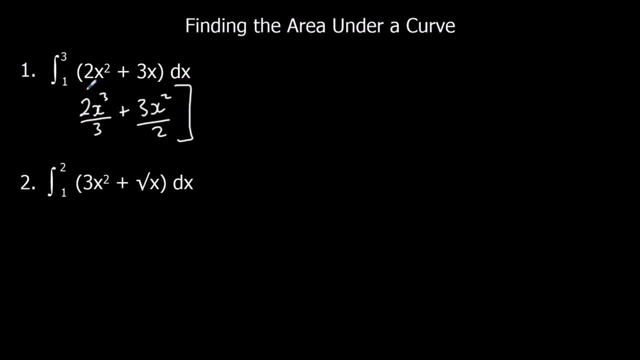 power divided by the new power. so we've got between 3 and 1 here. So substitute in 3, so 2 times 3 cubed over 3 plus 3, 3 squared over 2, take away 2 ones. 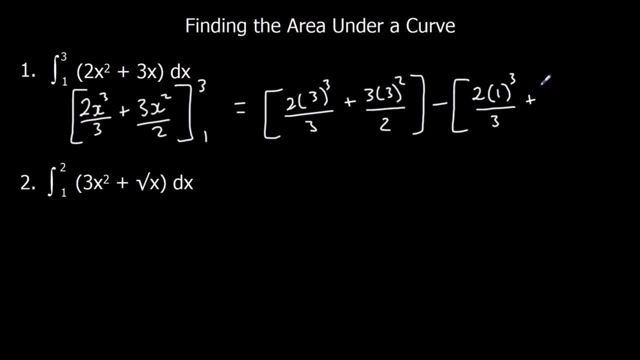 cubed over 3 plus 3 ones squared over 2.. Okay, then type it into the calculator And we should get 88 over 3.. Okay, second one here. so we're going to change root x to x, to the power of a half, and then 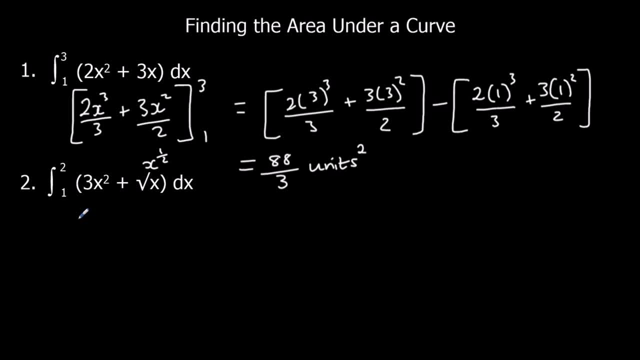 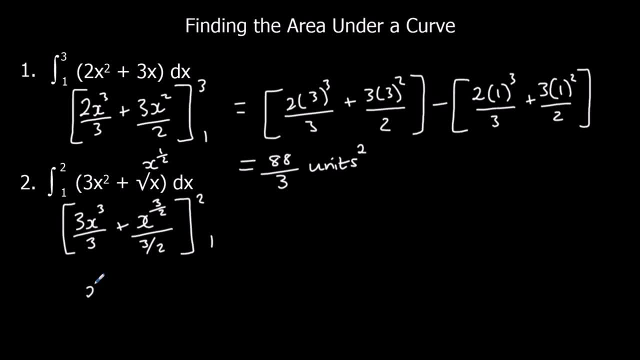 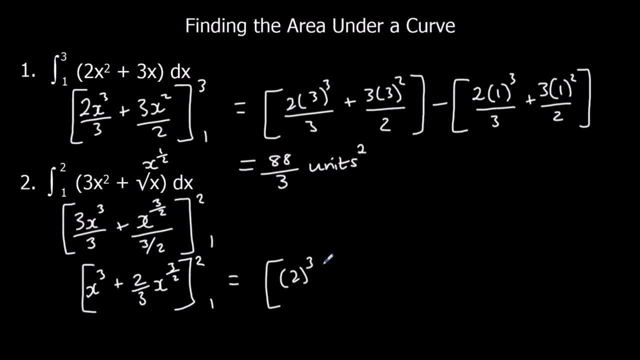 So we've got 2 cubed plus 2 thirds of 2, to the power of 3 over 2.. Okay, Okay, Take away 1 cubed plus 2 thirds of 1 to the power of 3 over 2.. 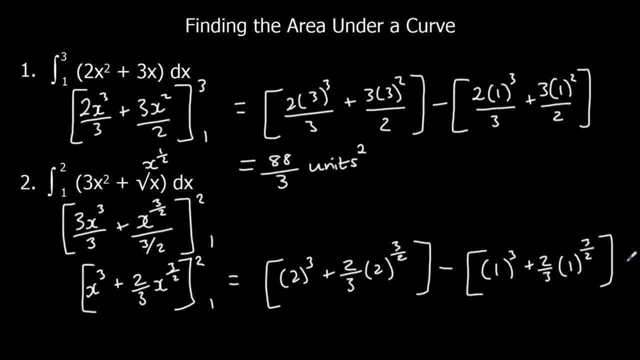 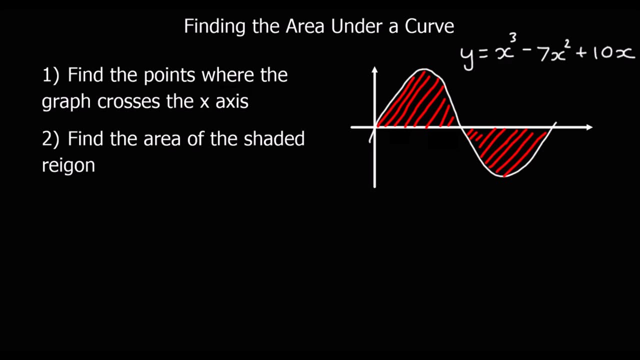 Type it into the calculator and that's giving us 8.22 to 3 significant figures and again units squared. So here we've got a more complicated question, because we've got part of the graph squared and then we've got part of the graph squared. 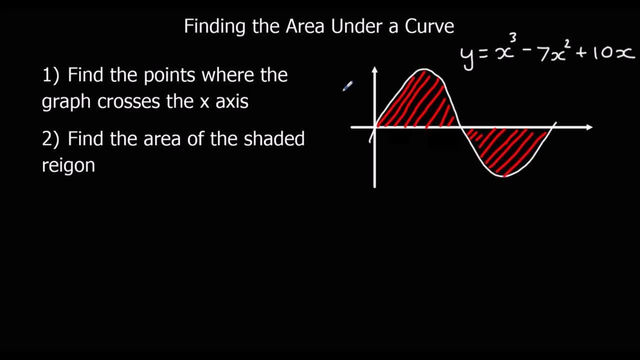 Okay, So we've got part of the graph above the axis and part of the graph below the axis, So we can't do this question in one go. The reason is this green area here. that will give us a negative answer. 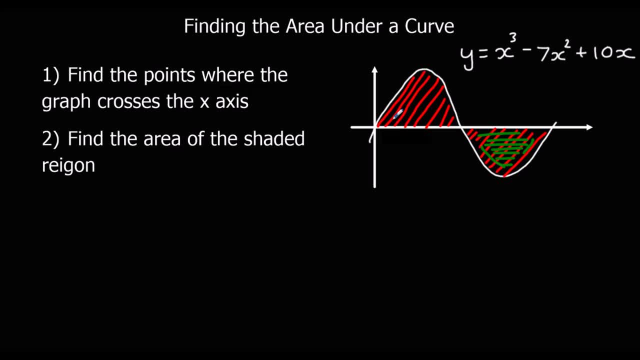 So below the axis it'll give us a negative answer And this purple area here will give us a positive answer. So if we try to do it all together, it would cancel out. So you'd have the positive bit, take away the negative bit. 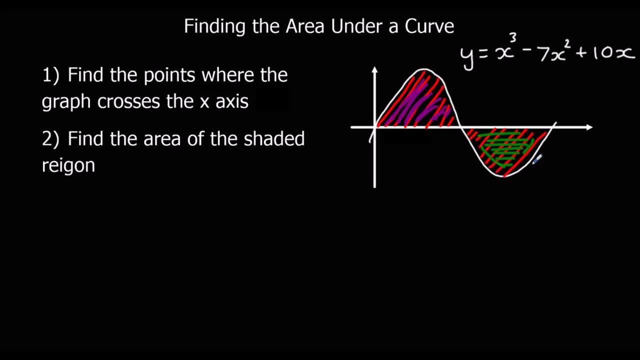 That's not what we want. We want all of it together. So whenever we've got a question like this with part of the graph above the x-axis, part of the graph below the x-axis, we need to do two separate bits. 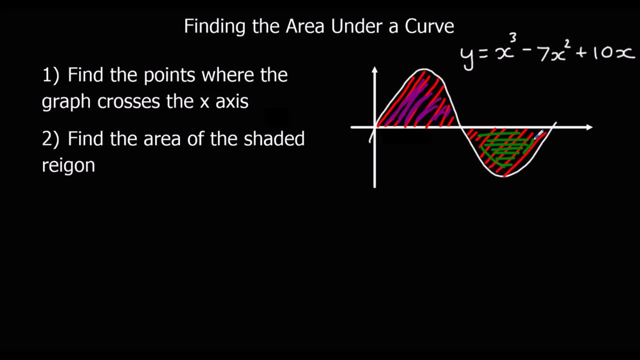 So we need to work out the area of the purple section, the area of the green section separately and add them together. So let's go through this question. So the first point is we need to find the points where the graph crosses the x-axis. 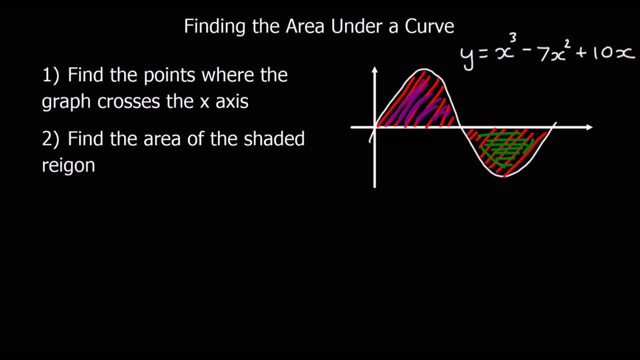 So it crosses the x-axis When y equals 0.. So we'll make y equal to 0 first, And then we will solve it by factorizing. So we'll factorize out an x first, And then we'll put the bracket into two separate brackets. 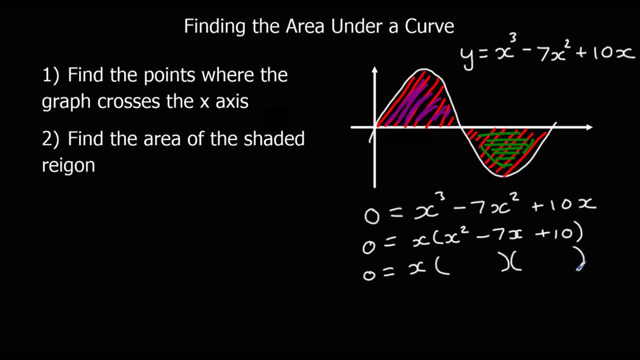 What multiplies to make 10 and adds to make negative 7. That will be x minus 2 and x minus 5.. So where does it cross the x-axis? It crosses at x equals 0,, x equals 2, and x equals 5.. 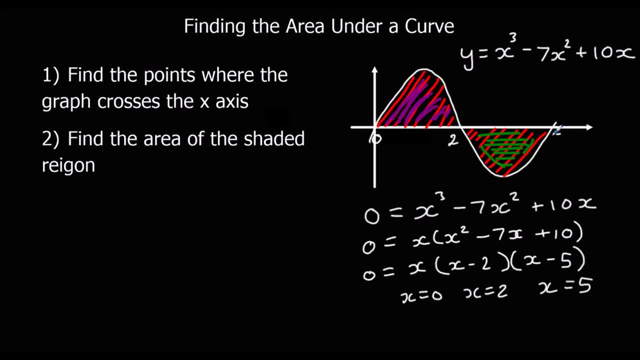 So we've got 0 here, 2 here and 5 here. So to find the area, the total area, the area of the shaded region, we're going to do two separate bits, Questions almost. So we're going to do the area in between 5 and 2.. 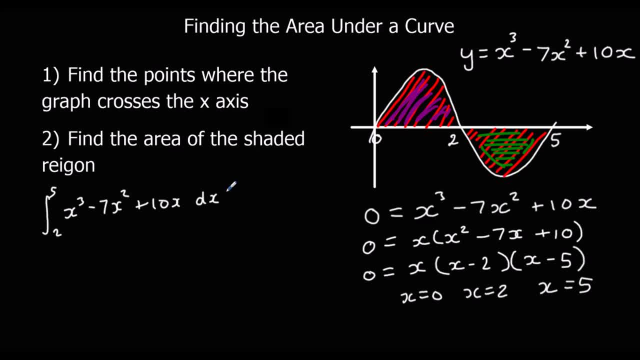 And separately we'll do the area between 2 and 0. So let's integrate this. So we're going to add 1 to the power divided by the new power. Add 1 to the power Divide by the new power. 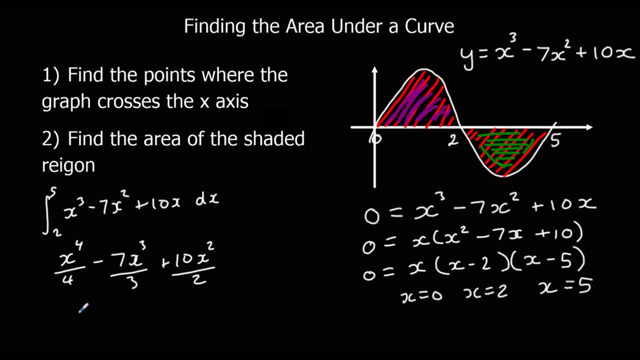 Add 1 to the power divided by the new power, And of course we can simplify that. so we'll go x to the power of 4 divided by 4 minus 7x cubed over 3 plus 5x squared, and that'll be between: 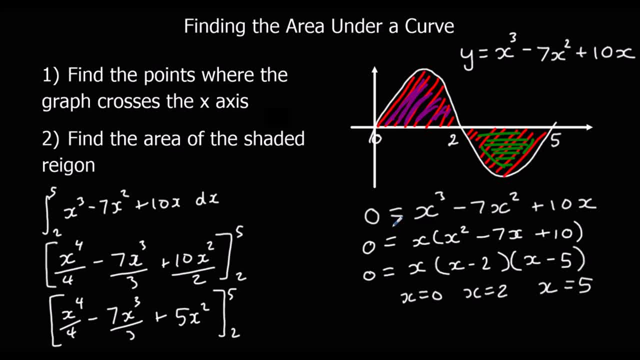 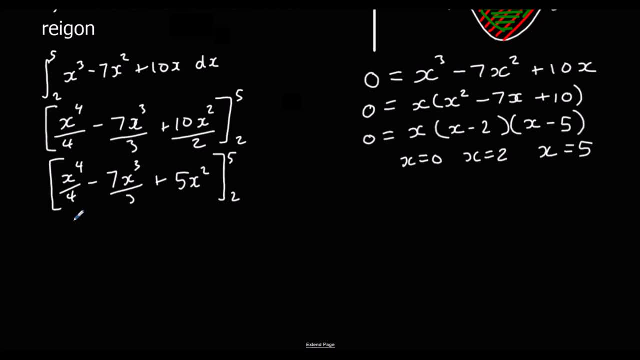 5 and 2 in the first instance. So we'll substitute in 5, substitute in 2, and take them away. So we've got 5 to the power of 4 over 4 minus 7 times 5 cubed over 3 plus 5 times 5 squared. 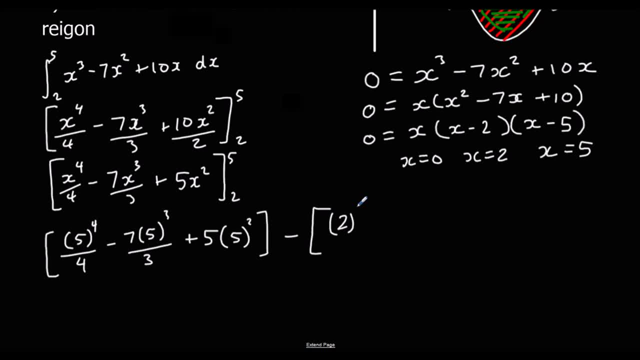 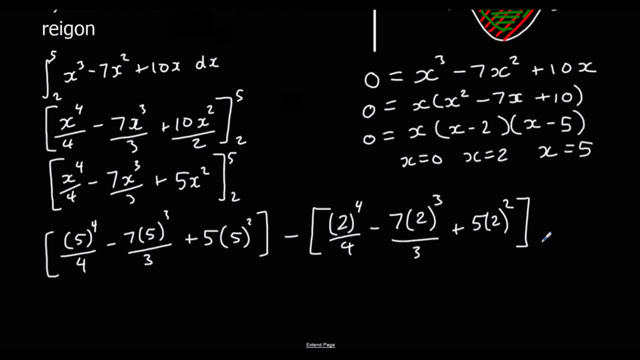 So we're going to type that into the calculator to see what we get out. And we should get minus because it's underneath the x-axis. so we've got minus 63 over 4.. Now we can't have a negative area. 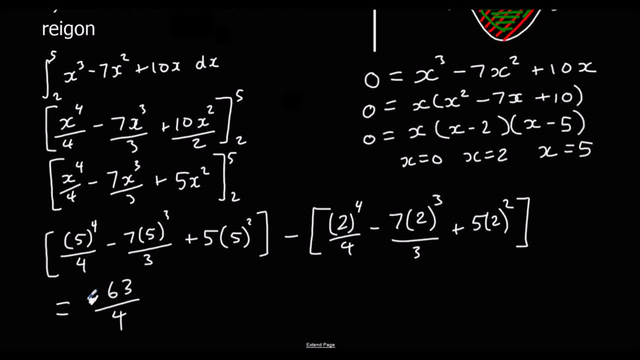 So we don't write the minus. so it's 63 over 4 units squared. So that's the green section, And then we're going to work out the purple section as well. So it's exactly the same thing, but instead of being between 5 and 2, it's going to be between 2 and 0 this time. 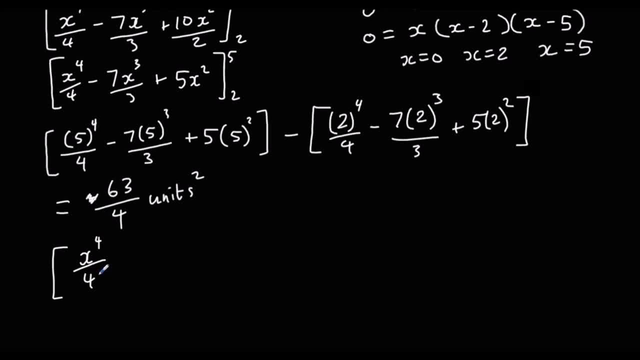 So So we've already integrated. We don't have to do that again. But this time we'll substitute in 2 and 0. Take them away And see what we get out. So if we type that into the calculator, we should get 16 over 3.. 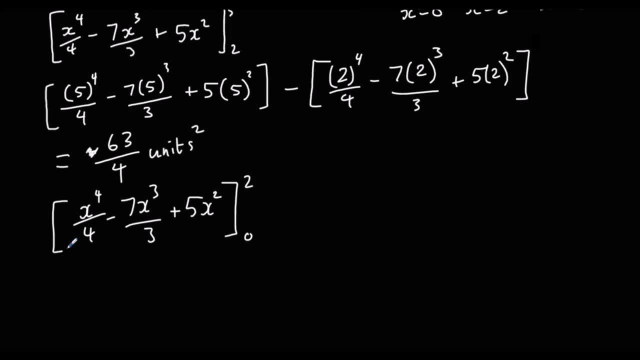 So I haven't written out that it's substituted in, So I will do that. So we've got 2 to the power of 4 over 4 minus 7.. So that's 1 times 2 cubed over 3, plus 5 times 2 squared minus 0.. 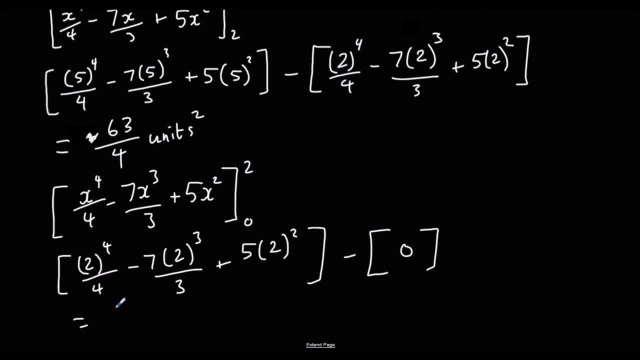 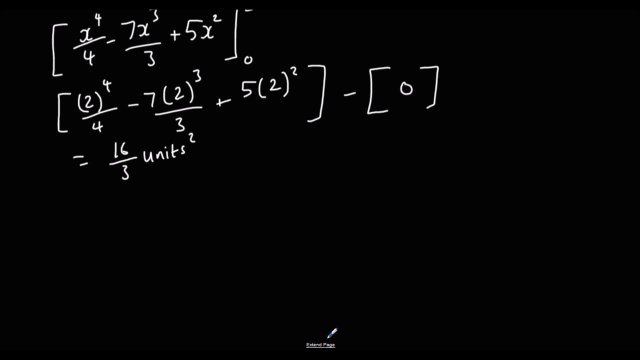 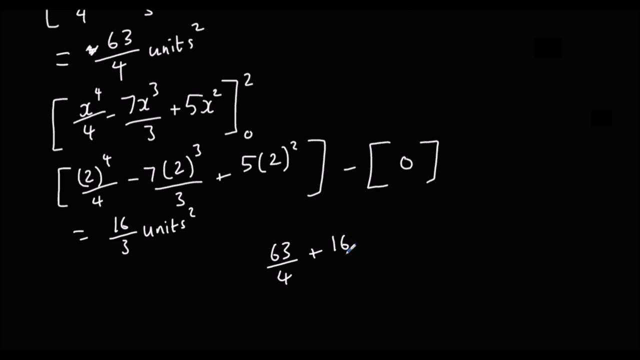 And then that should give you 16 over 3 units squared. So to work out the total shaded area. so we're going to add the green bit to the purple bit. So we've got 63 over 4 plus 16 over 3.. 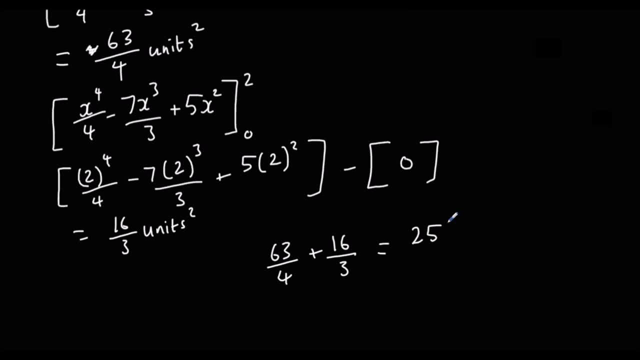 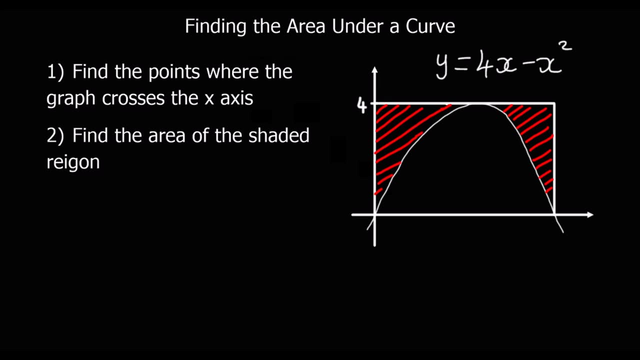 And that gives us 253 over 12 units squared. OK, another question here. So we've got Firstly find the points where the graph crosses the x-axis. So it crosses x and y is 0.. So 0 is 0.. 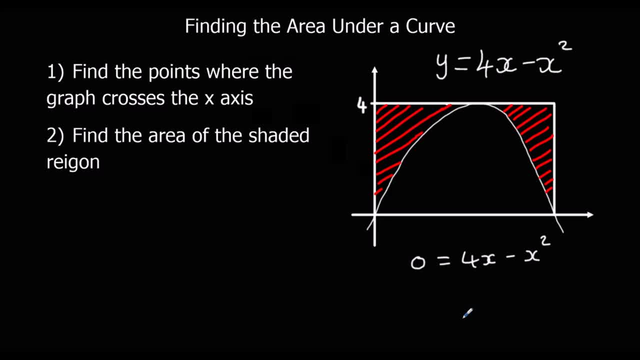 So 0 is 0.. So 0 equals 4x minus x squared. We're going to factorise it x 4 minus x, So x equals 0 and x equals 4.. So we've got 0 and we've got 4.. 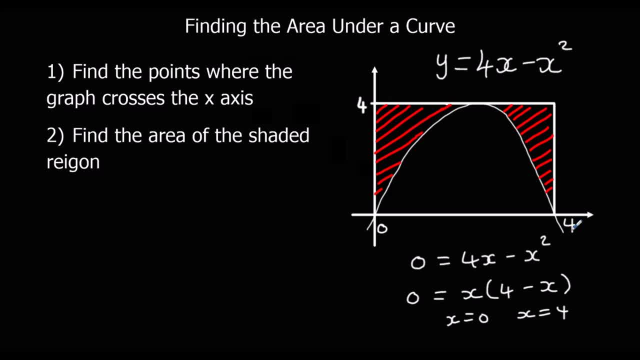 Find the area of the shaded region. So if we work out the area under the curve this time, that's going to give us this blue area here. So the shaded region is 0.. So the shaded region is going to be well, this square here. take away the blue area. 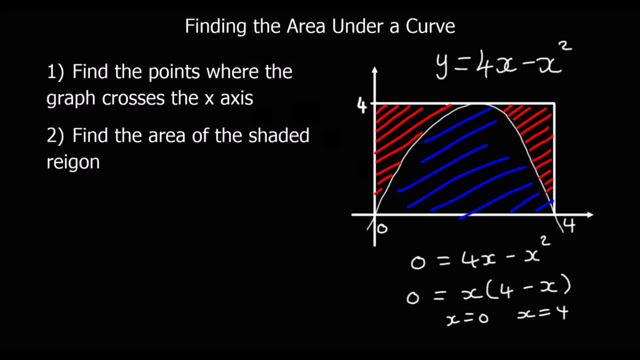 So the area of the square. So we've got a square which is 4 up, 4 along, So 4 times 4, that's going to be 16 units squared. So we're going to work out the area of the blue area, the area under the curve. 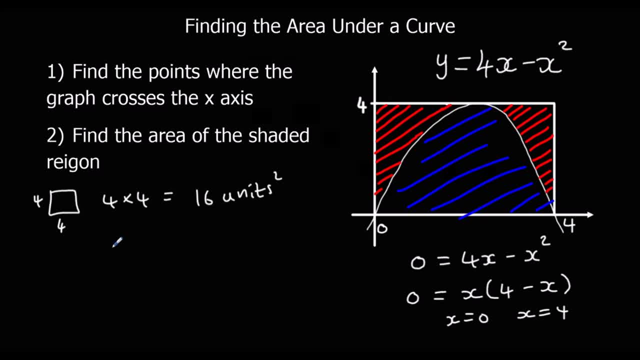 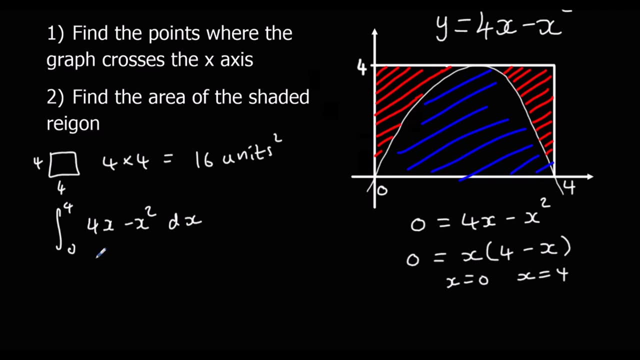 And then take it away from 16.. So we've got the integral of 4x minus x, squared between 4 and 0. So first step we're going to integrate. So add 1 to the power divide by the new power. 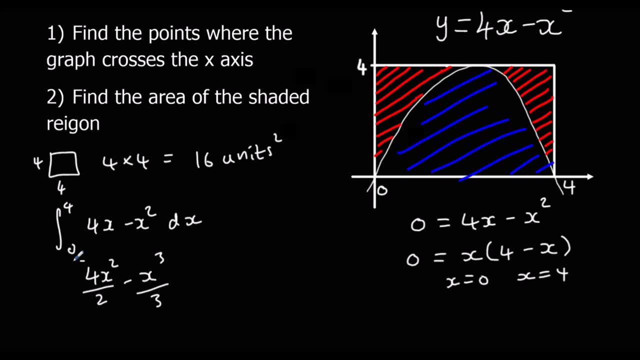 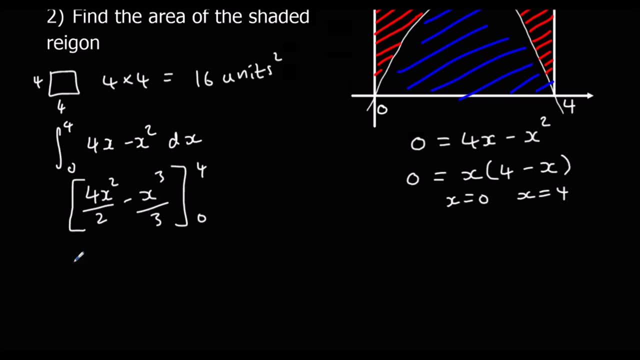 And add 1 to the power divide by the new power. So we've got 4. Between 4 and 0 this time. So we're going to substitute in 4. Substitute in the 0. And we're going to take them away. 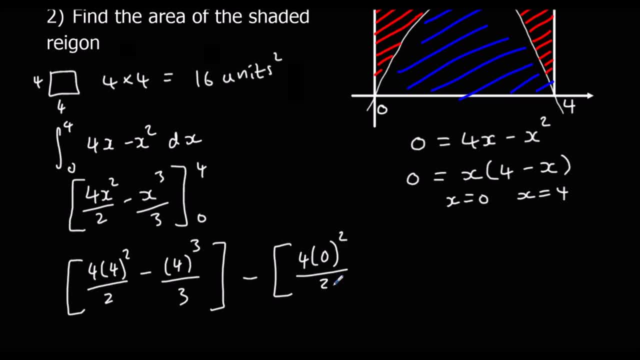 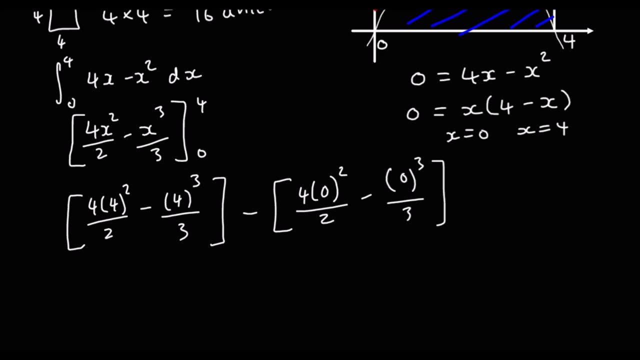 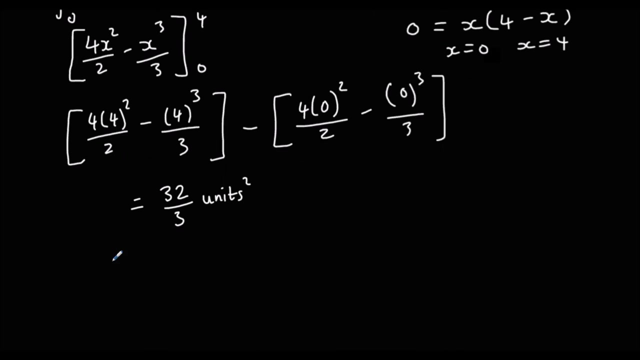 So we're going to take them away, So we're typing the calculator, So we're typing the calculator. So that gives us 32 over 3 units squared. But that's the blue area, remember. So the shaded region is going to be 16 minus that answer. 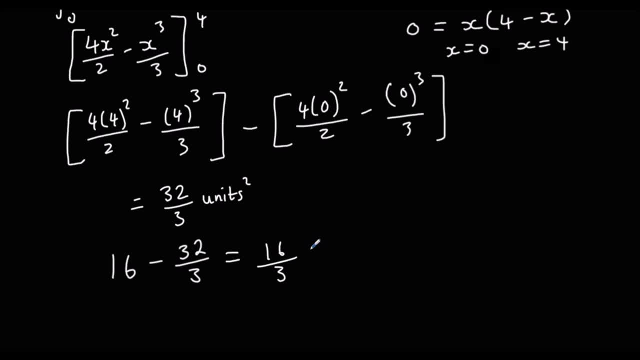 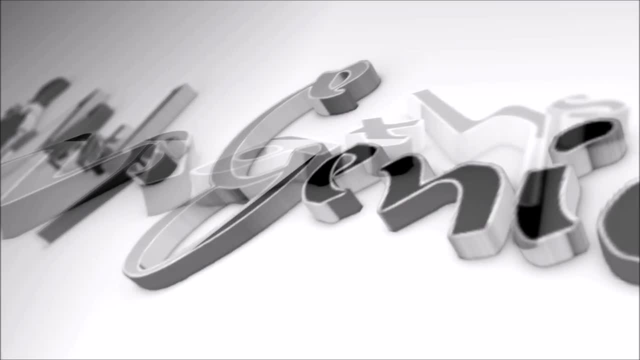 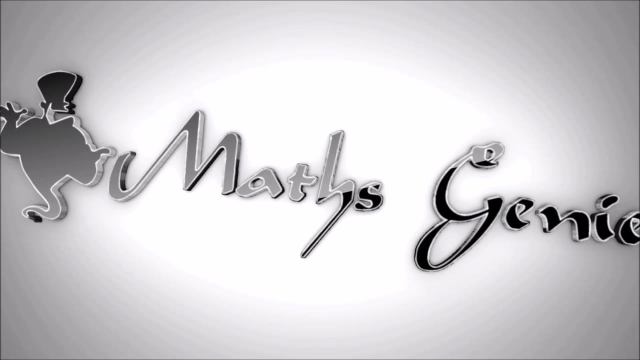 Which is 16 over 3 units squared. So we're going to plus that by 17.. So we'll call it black and times five. So move the neue r and I'll call it P. You're going to step back and pull the P over P's. It's the original number And I added the long, And we're going to put the dot mark where 9 and 8, and look at the blue and orange. we had alreadyGive that a try and figure out what we've got now. So in algebra what we've got is 8. �1 w, w1, w2, y1, w2, 0, 3. And we're going to export w1 to double the value, w1 to z.